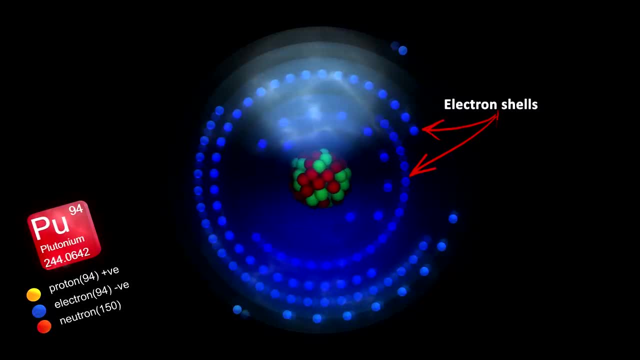 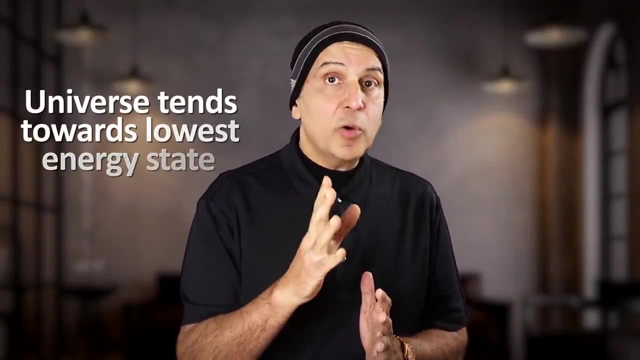 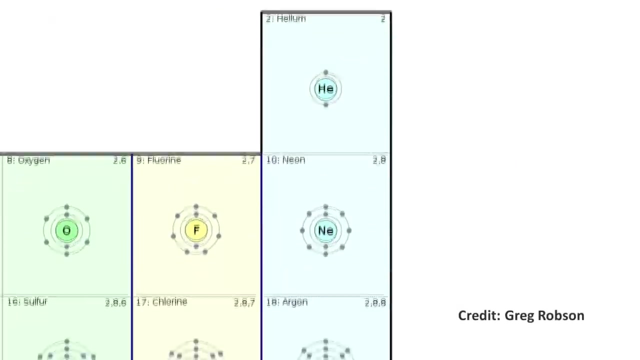 the Quantity of electrons in the atom, The universe tends to the lowest energy state. This applies to electrons. Some configurations of electrons are simply more energy efficient than others. It so happens that the lowest energy configurations of electrons is when the electron shells are either empty or full. What do I mean by shells? To explain this concept, 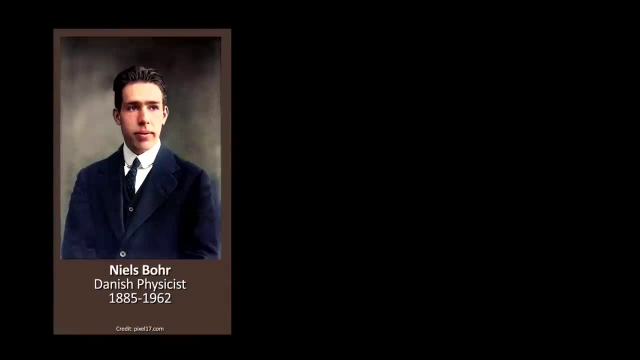 in a brief way. let's look at the oversimplified Bohr Model of the atom. Bohr'seremче model of the atom. Bohr'serem. UM2's central atom was formed when the electron shells were empty. Bohr'serem Exactly. 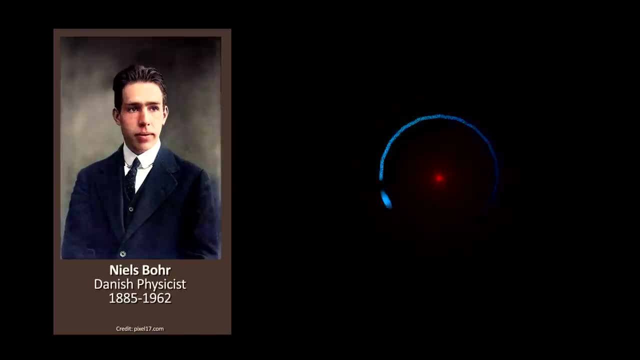 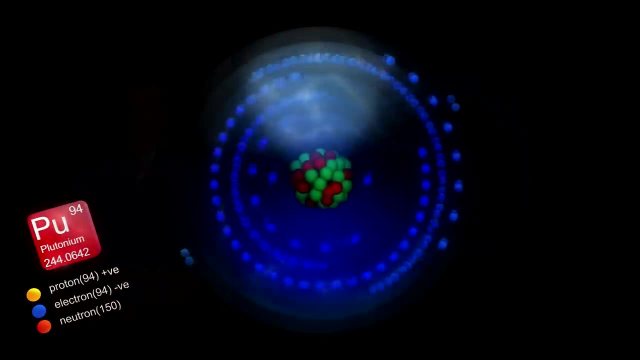 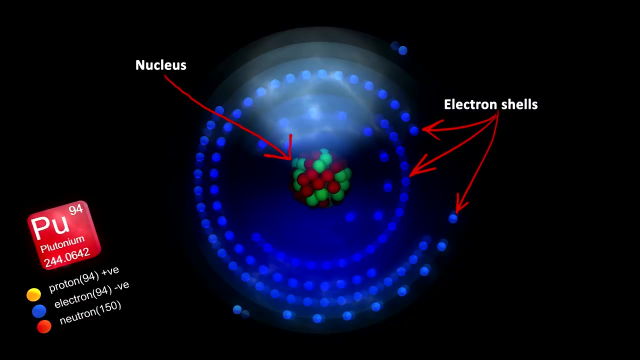 Bohr showed that electrons can only exist in certain stable orbits around a nucleus where the angular momentum is proportional to Planck's constant. These are like shells around the nucleus. We can draw the atom where the nucleus is in the center and the rings around it represent the electron orbits, or shells. 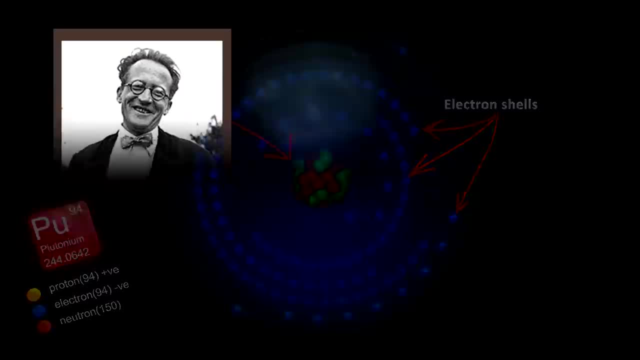 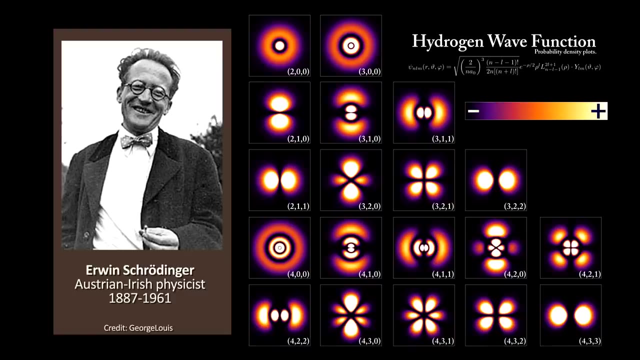 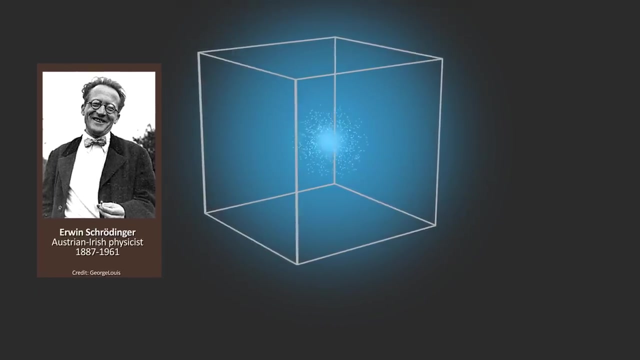 But this model, of course, was an oversimplification. Erwin Schrödinger understood that, rather than being confined to an orbit like a planet, an electron is a matter wave that forms a probability cloud in 3D space, smeared around the nucleus according to quantum mechanics. 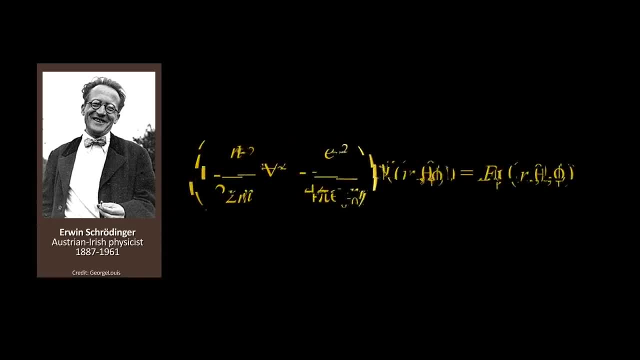 And he formulated the rules to describe this behavior, the famous Schrödinger equation. This equation, as it turns out, went beyond the Bohr model of the atom by more accurately describing every atom that exists in nature, In other words, the structure of the entire. 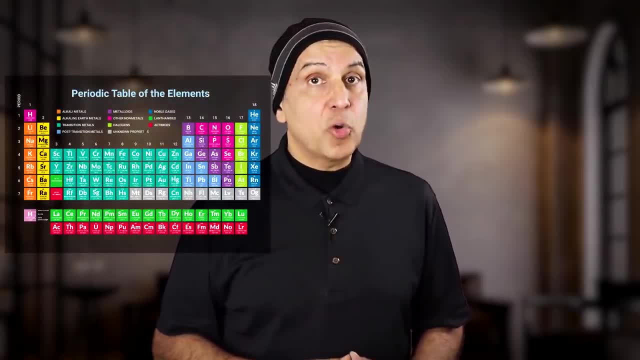 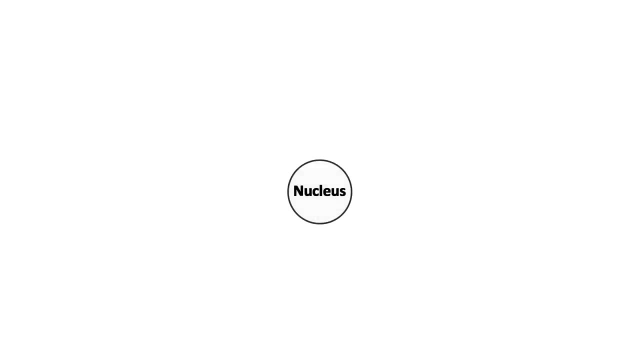 periodic table of the elements, Electrons can be predicted by Schrödinger's equation. This was nothing short of astounding. The Schrödinger equation showed that each shell has a maximum number of electrons it can hold. The innermost shell holds a maximum of 2 electrons. The second holds a maximum. 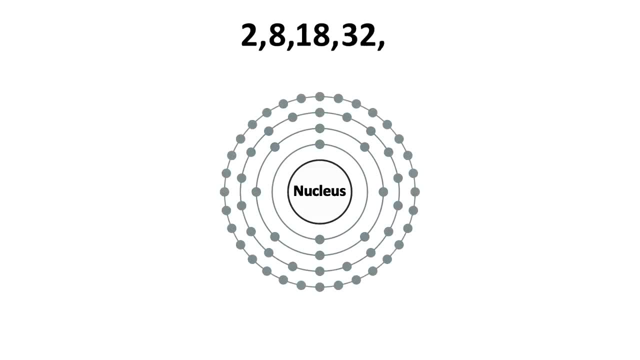 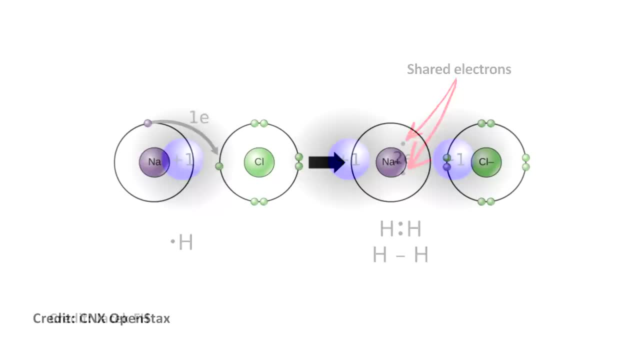 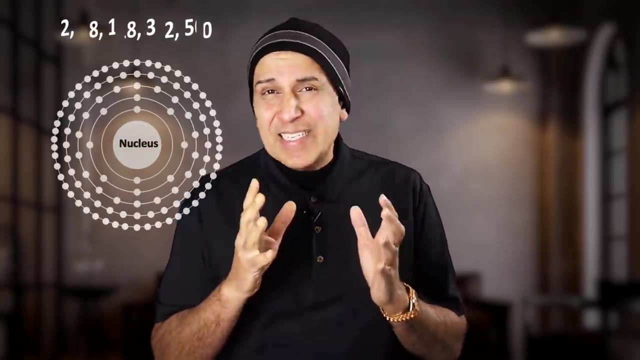 of 8 electrons, The next up to 18,, then 32,, then 50,, and so on. Chemistry is about substances exchanging or sharing electrons in order to fully fill up these shells. Okay, so now the elephant in the room that needs explaining is: why are these numbers? 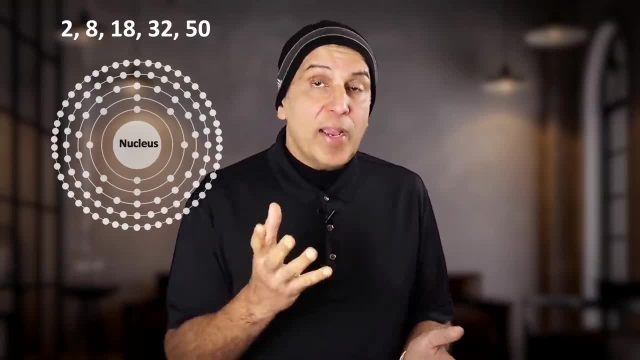 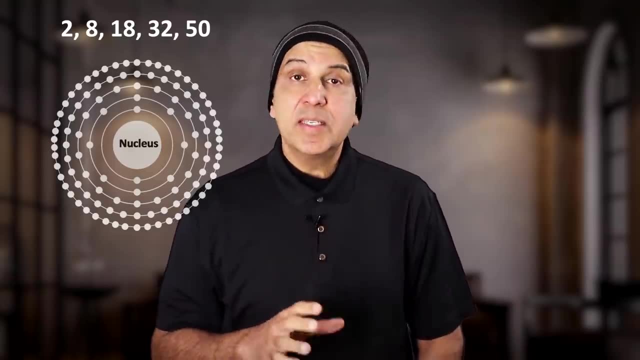 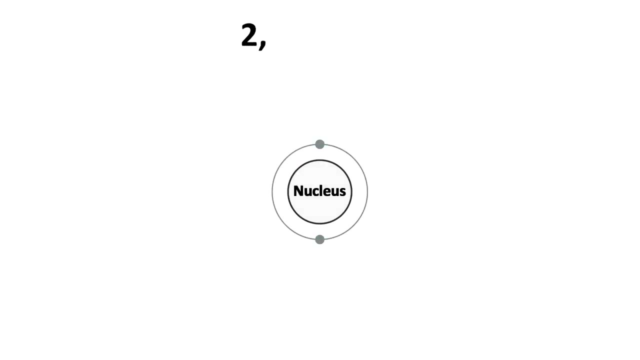 so special These numbers look random. Why in the world do atomic interactions care about conforming to these numbers? It all comes down to energy. Systems in the universe tend towards their lowest energy state. To minimize energy, the electrons fill up the orbits, starting from the center and 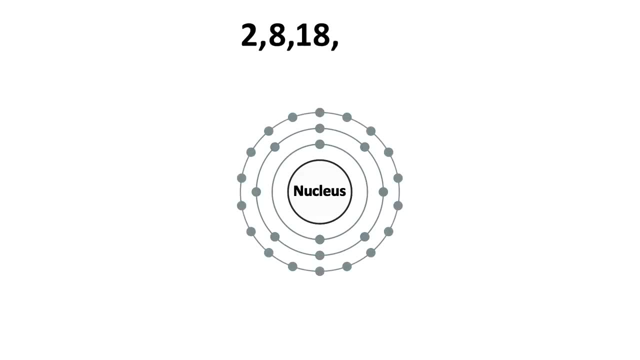 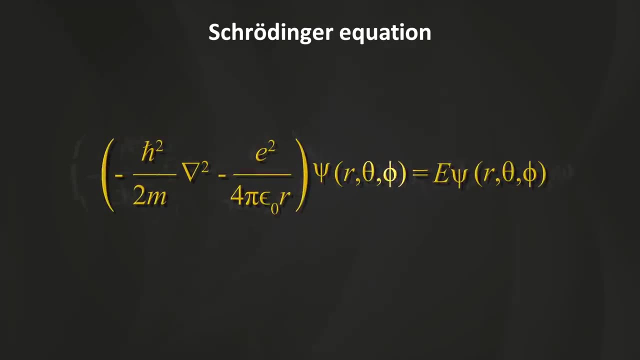 moving out. This minimizes the energy of the atom. To understand why we have to solve the Schrödinger equation. Although this equation looks intimidating- and it can be- in its essence it's just a statement of energy conservation. It simply. 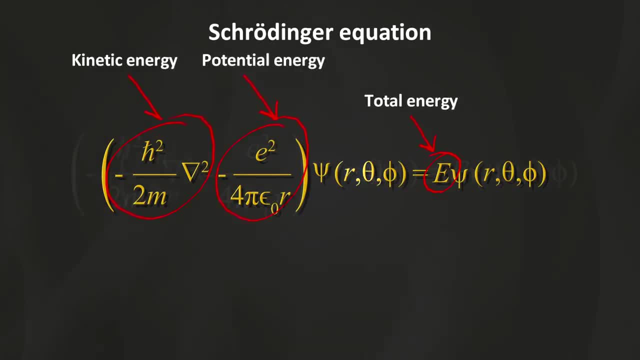 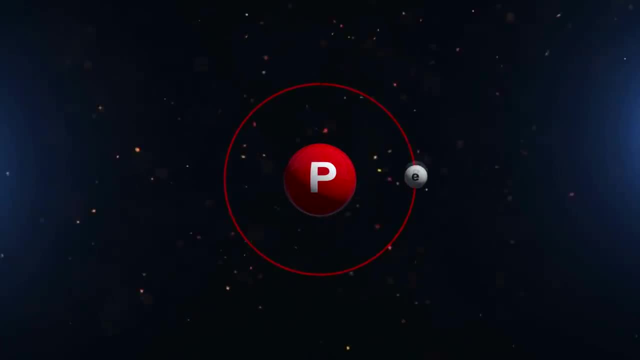 says that total energy is equal to potential energy plus kinetic energy. That's it. This equation can be solved most easily for the hydrogen atom, because it is the simplest atom: Just one electron orbiting one proton. Because the core is made of just one proton, it's spherically symmetrical. 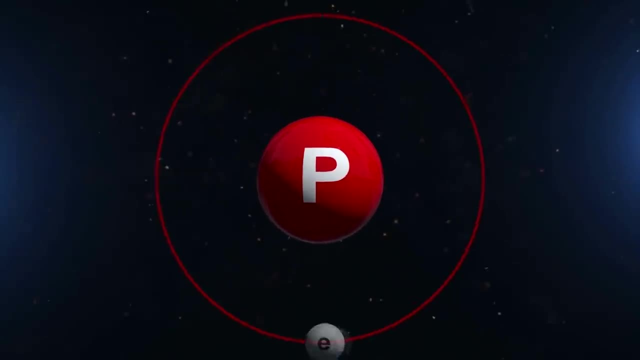 If you imagine the proton like a ball, it doesn't matter how you rotate it, It always looks the same. It has symmetry. If we consider something like hydrogen-2, also called deuterium, which has a proton and neutron in the nucleus, it would no longer be spherically symmetrical. 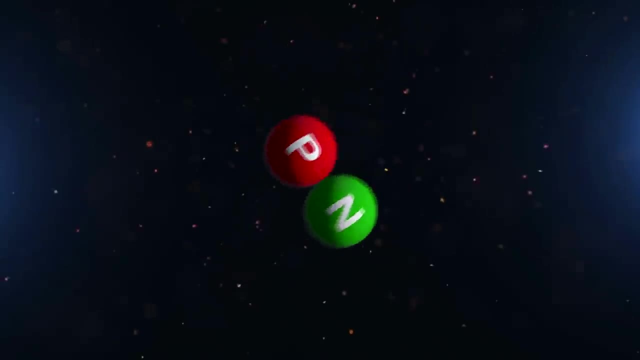 because if you rotate the nucleus, the neutron would point in a different way. This spherical symmetry is essential for making the solution simple enough to solve the Schrödinger equation exactly Now. I don't want you to get intimidated by this equation, I just want you to get familiar with it. 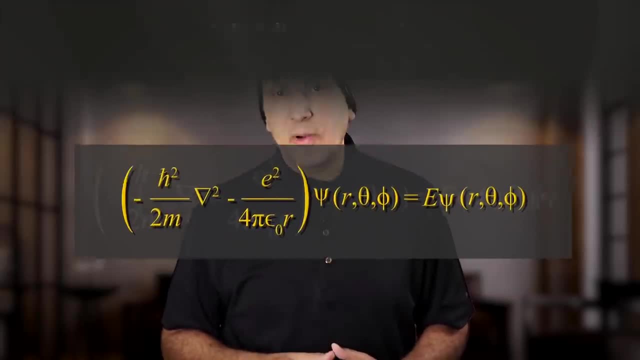 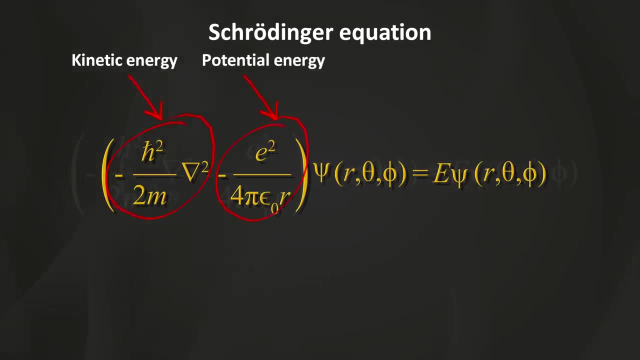 so that you can understand where the electron shell numbers are coming from. In the Schrödinger equation we have a kinetic energy term and a potential energy term that we define Because hydrogen has a positively charged nucleus and a negatively charged electron. 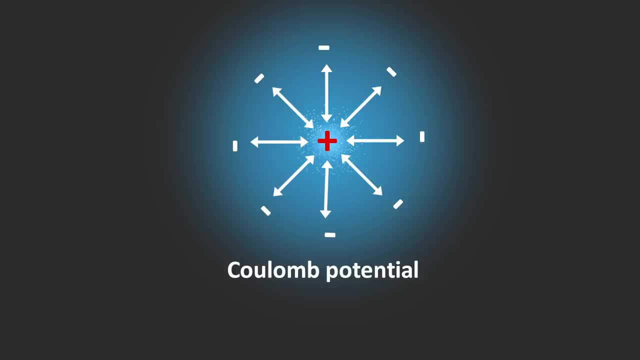 there is an attractive Coulomb potential between the electron and the proton. This is where the potential energy term comes from. There are several constants in this equation. There are several constants in this equation. There are several constants in this equation. The площadht key is P. the relative momentum of the atom, the control volume of the atom. 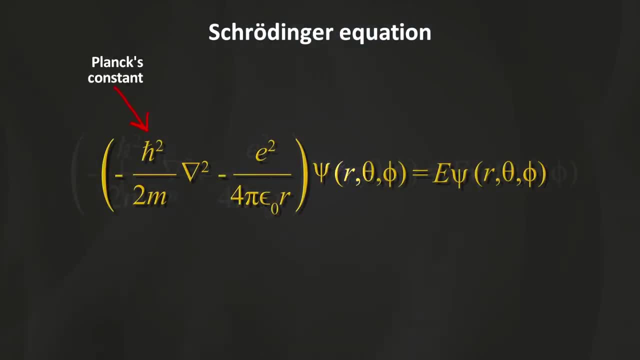 theni-y function of the atom and the voluntary charge function of the atom. We can use theійc constant to solve the equation which we don't have to solve for, as shown here, Planck's constant, epsilon, or the vacuum permittivity, the mass of the electron and proton. 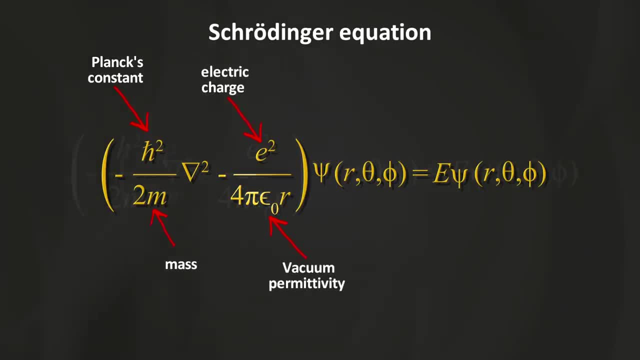 and e the electric charge constant. I won't derive this equation in this video because that's not important for understanding the subject we're covering today. The key term to look at here is psi. This is the term we have to solve for. 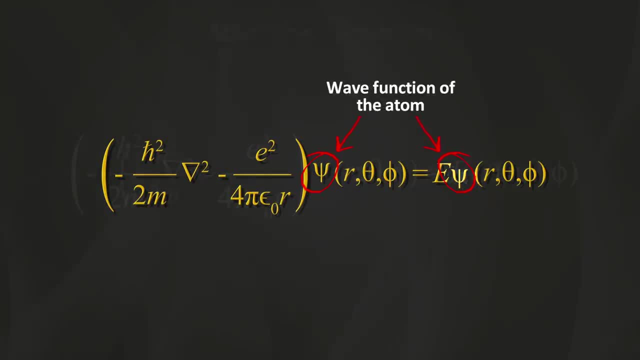 It is the wave function of the hydrogen atom. It represents a value that is related to the probability of this atom being, in a certain way, Rock-Style. However, we don't know the difference between a negative and negative value. This is why we're looking at this equation. 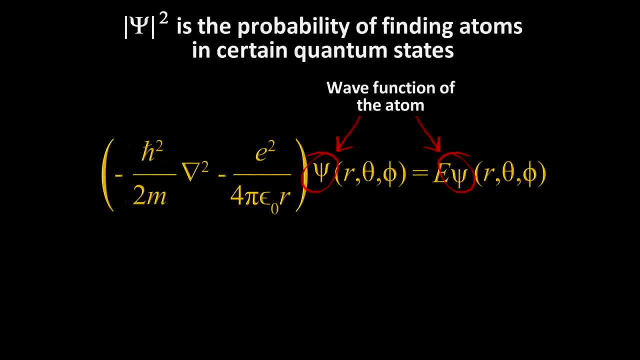 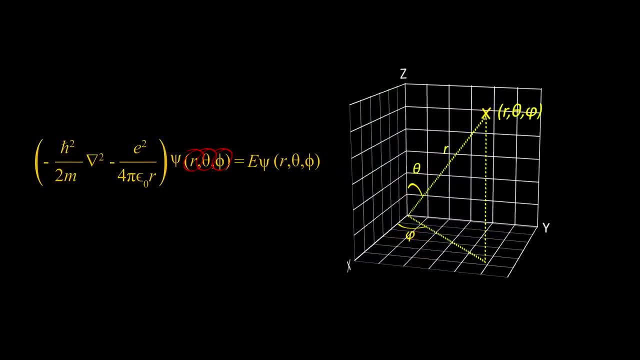 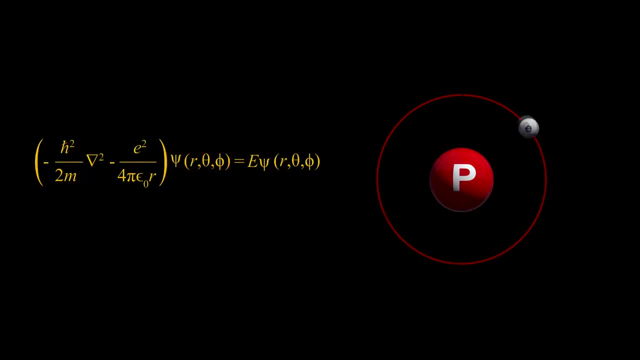 of this atom being in certain quantum states, The radius and angles. theta and phi represent the spherical coordinates of our system in three-dimensional space. Now, even though this is the simplest atom to solve for, it's still quite difficult to do. But solving for the wave. 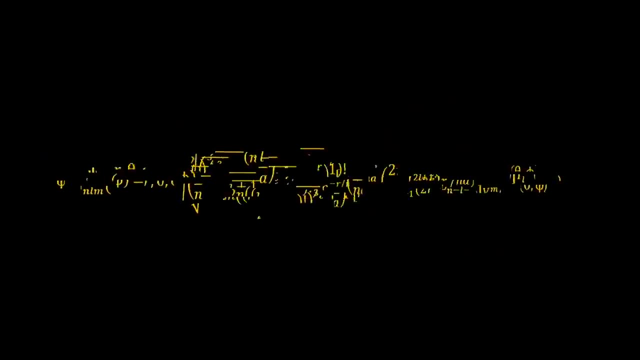 function of the hydrogen atom gets you the following result: This equation is a bit of a mouthful and it takes many pages and hours of work to derive, but let's look at some of the components so that you can understand how this plays a role in the shells around the nucleus. 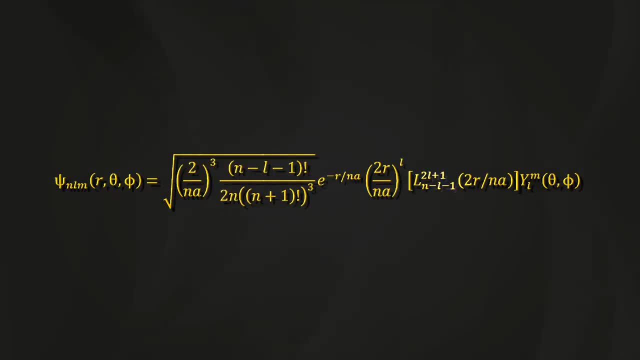 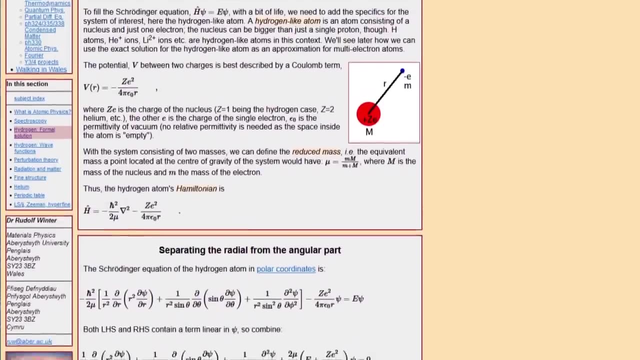 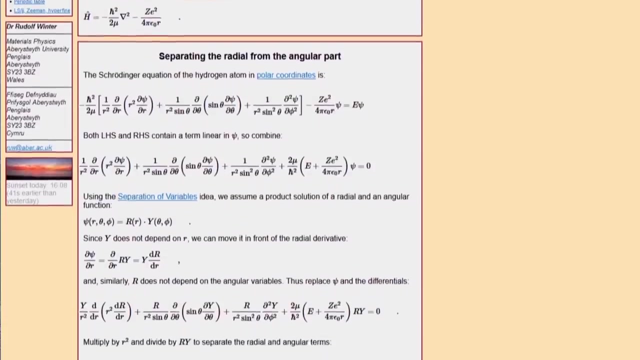 The main thing I want you to look at are these three extra labels N, L and M. Where did these come from? When solving the Schrodinger equation, you get a set of complicated differential equations. In order to solve these, you have to specify some quantum values for the atom. These are values or? 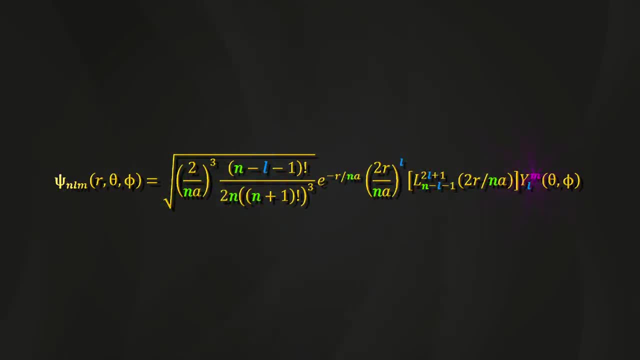 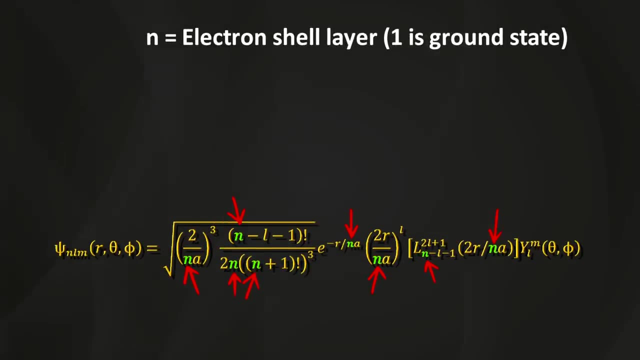 quantities that have to be inserted in the equation to solve for psi. I have a link to the long solution if you want to see how this is done. N just represents the electron shell layer. N equals one, is the ground state or the lowest energy state of the hydrogen atom. 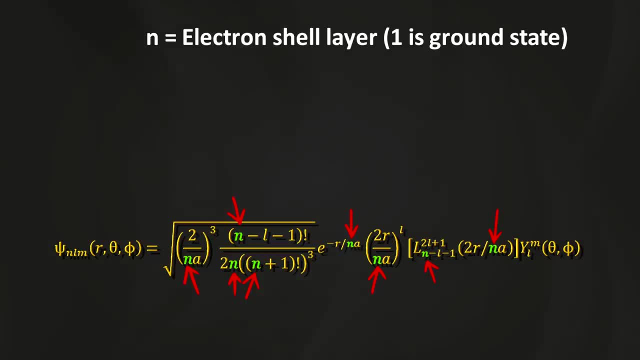 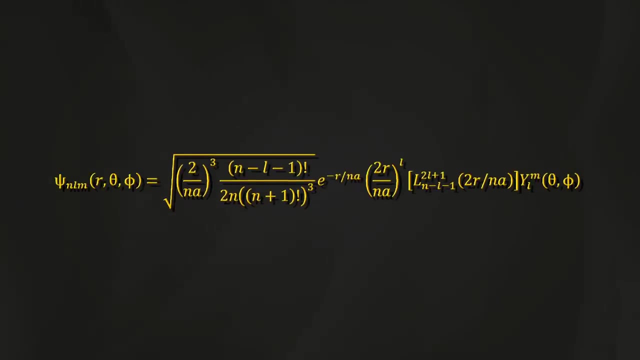 But hydrogen is not always found in its lowest energy state, so it can take on other values. L is a quantum number defining the orbital angular momentum, And M is the number which specifies the orientation in space of the orbital. Now here's the key to the significance of this equation. 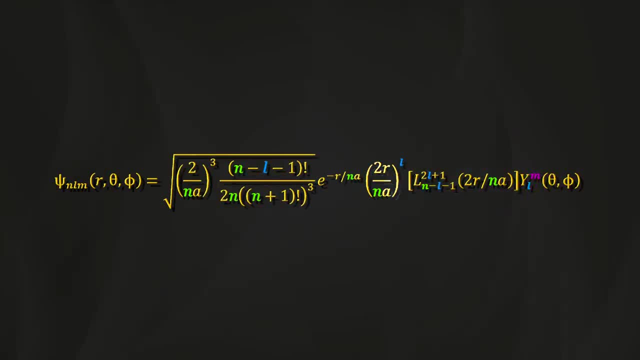 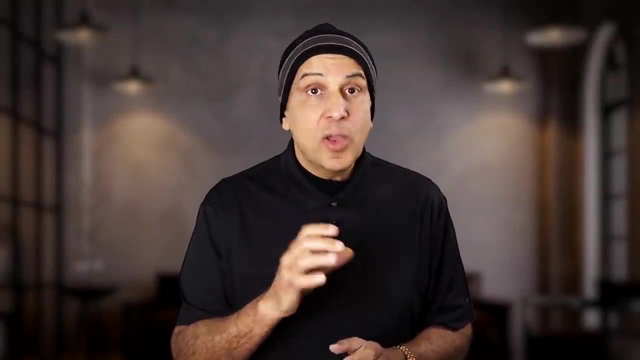 When we plug in different values for N, L and M in the Schrodinger equation for the hydrogen atom. it also approximately represents the solution to all the quantum states of electrons for any other atom. So this equation allows us to predict how electrons behave for all the elements of the periodic table. 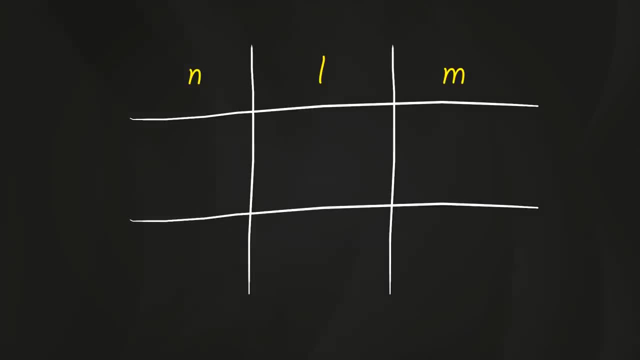 Now there are some rules for choosing the numbers. N must be an integer, starting with 1.. Since it specifies the shell. there is no such thing as a fixed magnitude or an infinite magnitude. The equation has to be taken into account. What you can do in the next few slides is to use these numbers. 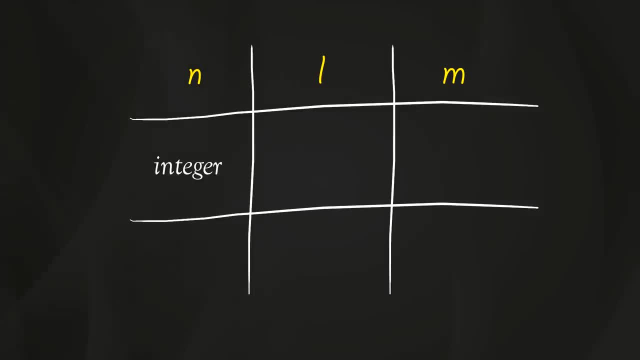 is no such thing as a 1.5 shell or 1.3 shell. the shells can only be 1,, 2,, 3, and so on. Depending on the value of n, l will be an integer from 0 to n-1.. And finally, the value of m depends. 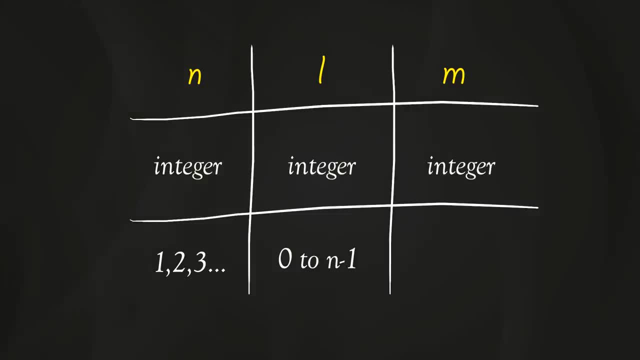 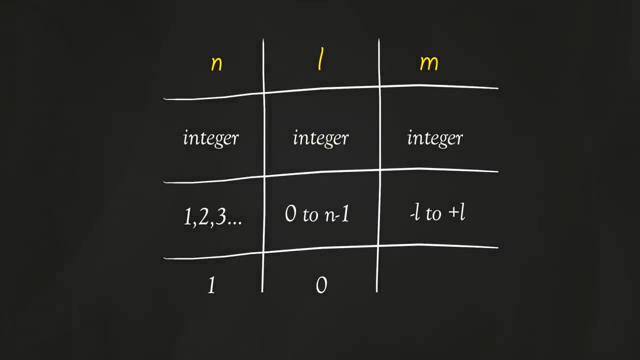 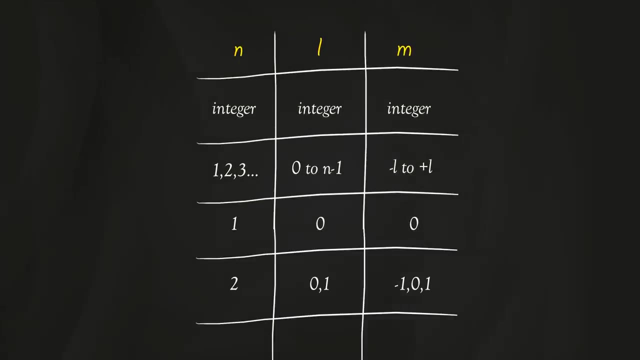 on the value of l. This can be integer values between negative l and positive l. For example, if n equals 1,, then we must have that l equals 0 and thus m equals 0.. If n equals 2,, l can equal 0 or 1.. And m can equal negative 1,, 0, and 1.. If n equals 3,, then we can have: 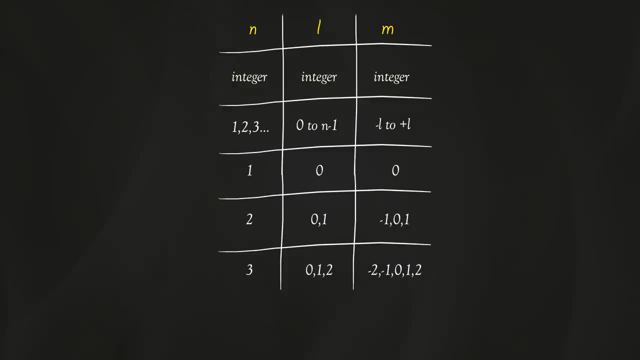 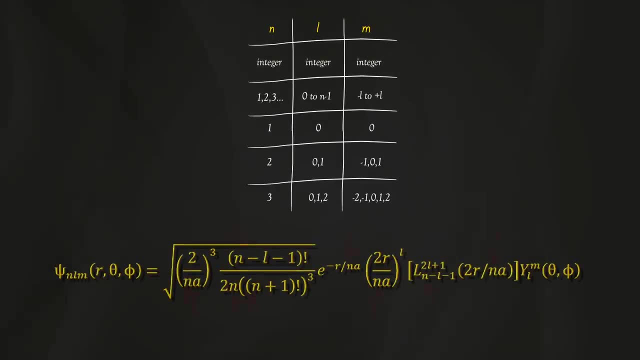 l equal to 0,, 1, or 2.. And m equals negative 2, negative 1,, 0,, 1, and 2 in that case. And this pattern continues. Now let's try to visualize it. Let's consider the case where 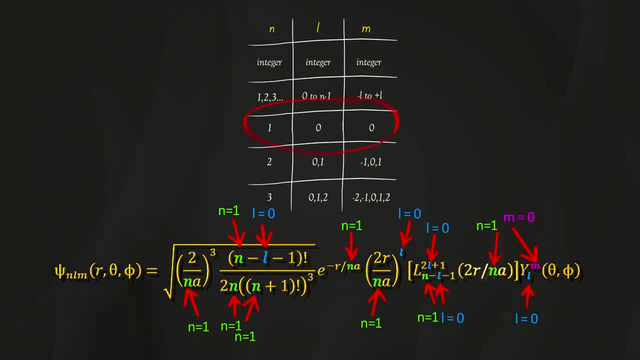 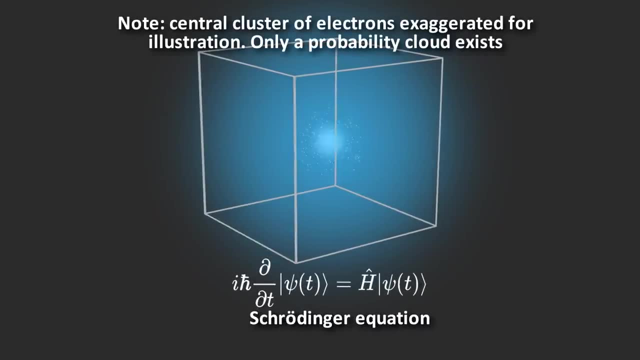 n equals 1.. This is the atom a, its ground state, l and m are zero. In this case, the result is a spherical wave function. It's just like a small fuzzy ball. The Schrodinger equation in this case indicates that the 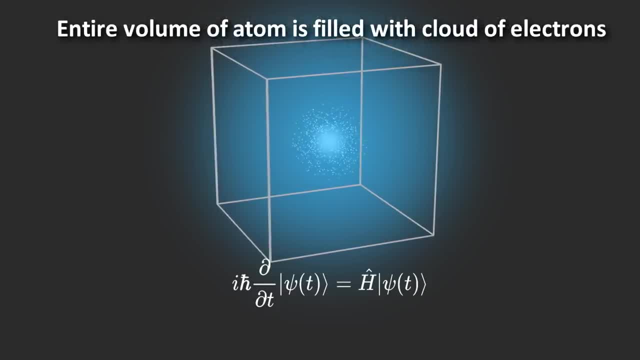 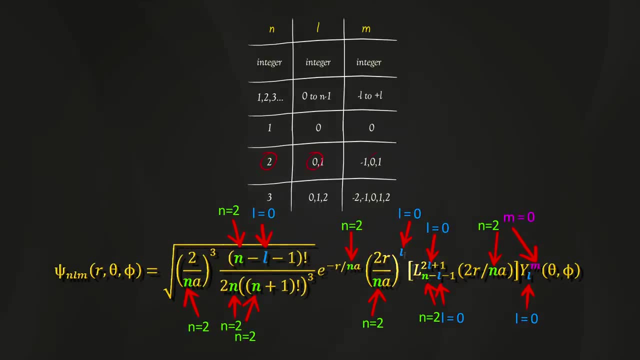 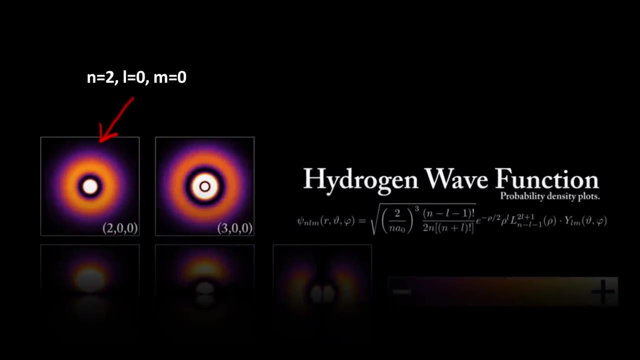 probability of finding the electron is in a spherical cloud around the nucleus. What if we solve for the case where n equals 2, a higher shell, and l and m are still both zero? In that case, the atom would be adding another shell around the first shell. In fact, if we keep 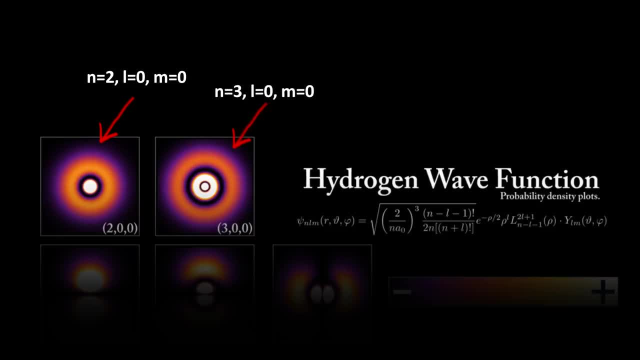 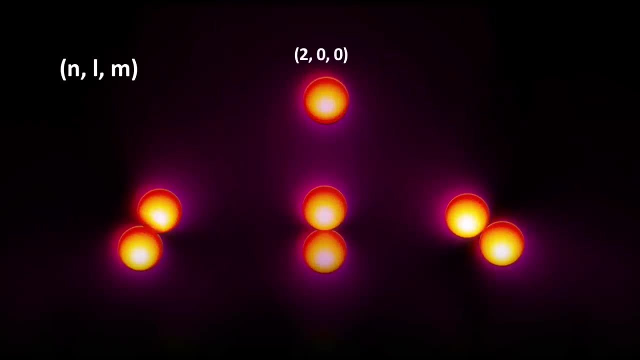 m zero, then as we consider n equals 3,, 4, and so on, we just add more shells around the nucleus. Now what if we set n equals to 2?? Keep l equal to 0, like before, but also l can equal 1.. 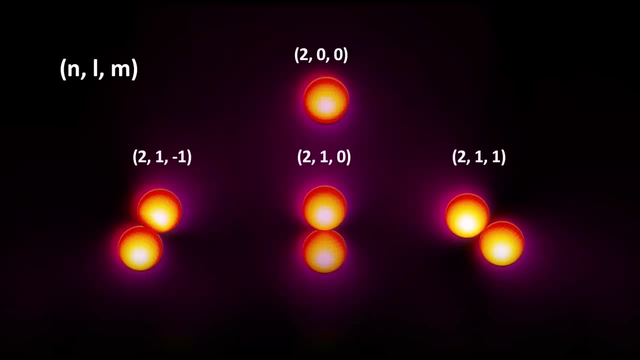 In the latter case, m can be either negative, 1,, 0, or 1.. Thus we would have one configuration with l equal to 0 and three additional configurations with l equal to 1.. So if we add all these configurations, we would have: 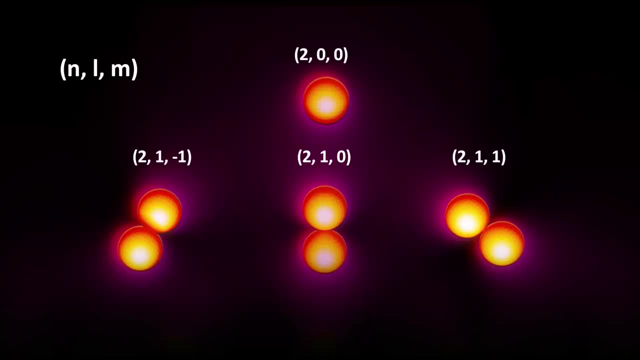 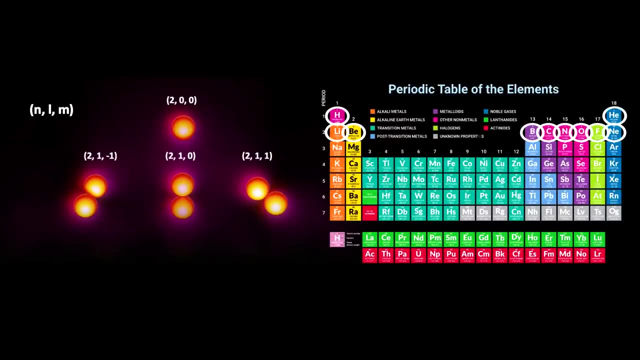 total of four configurations for the case where n equals 2.. Let's now compare this to the rows of the periodic table. The first row has two elements and the second row has eight elements. If n equals 1, we know that we can have one configuration. 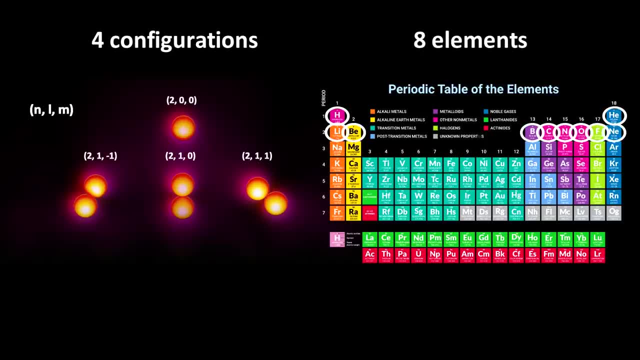 And if n equals 2, we know that we have four configurations. This looks similar to the possible electron shells in the atom, except that it's double: 8 instead of 4, and 2 instead of 1.. It turns out that these quantum numbers are explaining the possible shells. 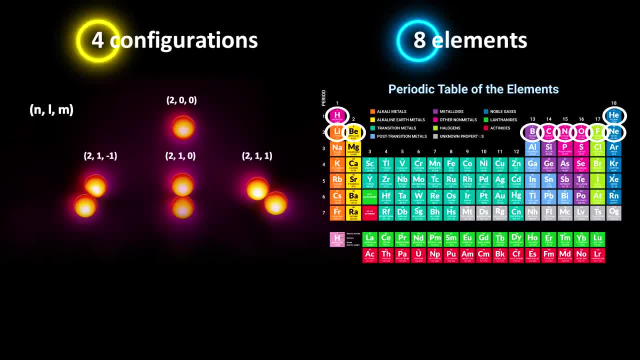 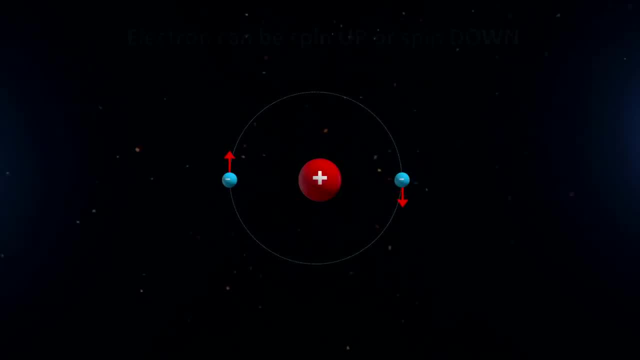 or orbitals available to the electrons. But then what about this factor of 2?? Where does this come from? Here's where you have to remember that electrons are spin one-half particles. This means they can be spin up or spin down. 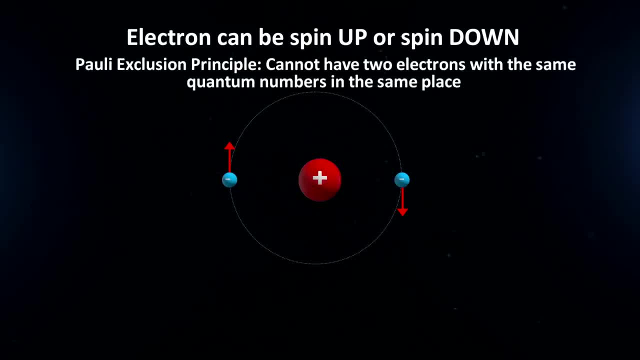 The Pauli exclusion principle says that you can't have two fermions. The fermions are electrons, in this case with the same quantum numbers in the same place. But you can have a spin up or spin down, And spin down for each choice of n, l and m. 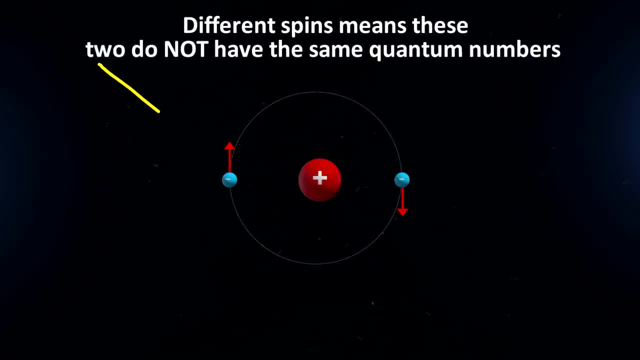 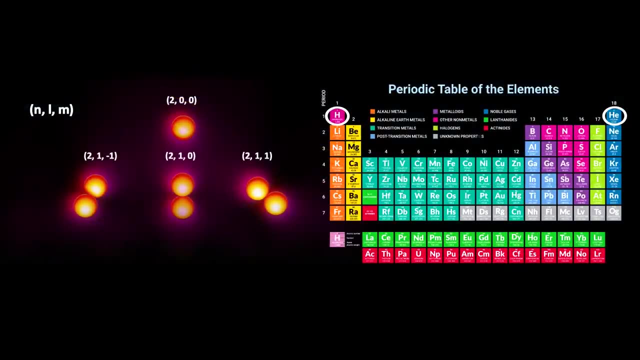 And because the spins are different, they would not be identical. This is why we have two electrons per configuration. So although the Schrodinger equation shows four configurations for n equals 1 and n equals 2, we can double it to eight configurations, since we can have four electrons with spin up. 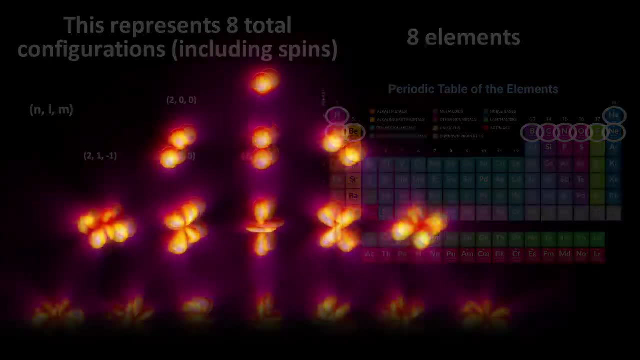 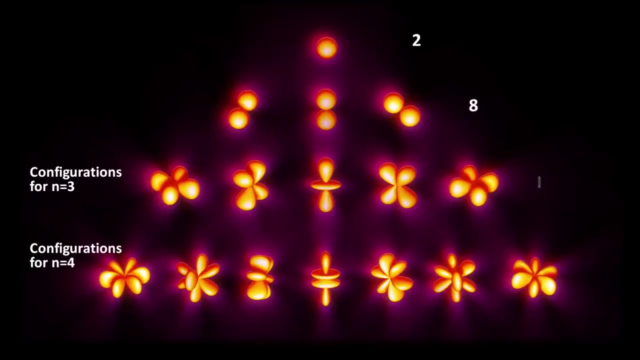 and four more electrons with spin down. Similarly, if we solve for n equals 3,, n equals 4, etc, we find that the total number of configurations is equal to the electron shell numbers I showed at the beginning of the video. 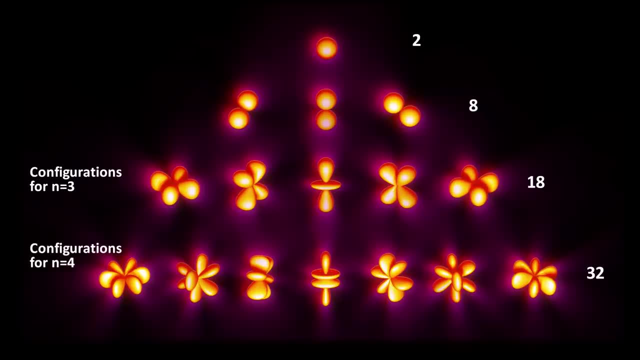 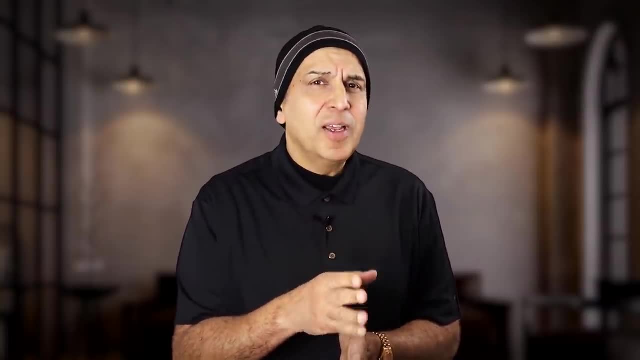 So the structure of the periodic table can be understood just by solving the Schrodinger equation for the hydrogen atom. But you might ask, why don't we need to solve the Schrodinger equation for helium or sodium or uranium to be really sure that the orbits are correct? 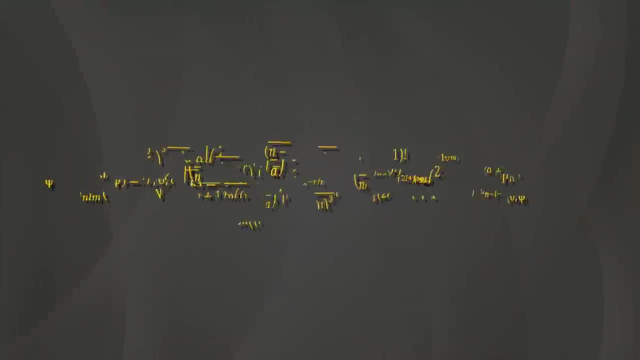 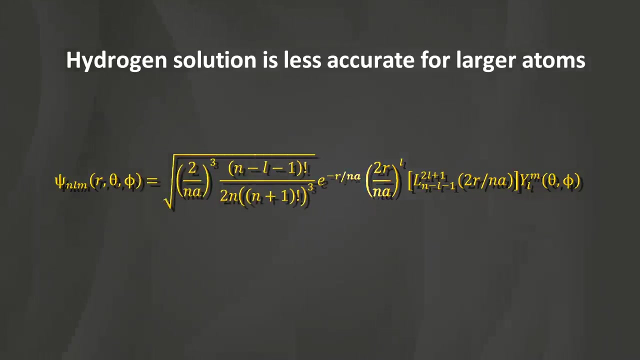 Can the hydrogen solution really work for all atoms? Well, the answer is no, not quite. This hydrogen solution isn't exactly correct. It gets less accurate. It gets less accurate for larger atoms. So if you look at it in detail, there's some small variations for the larger atoms. 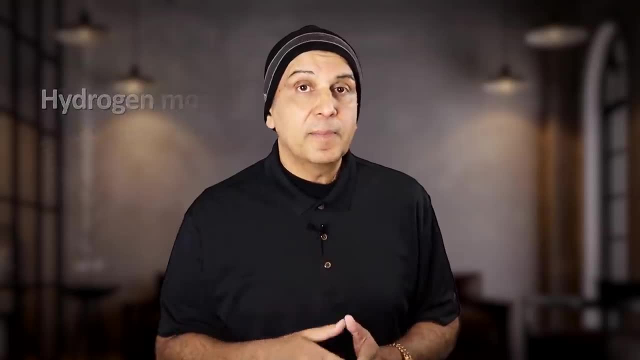 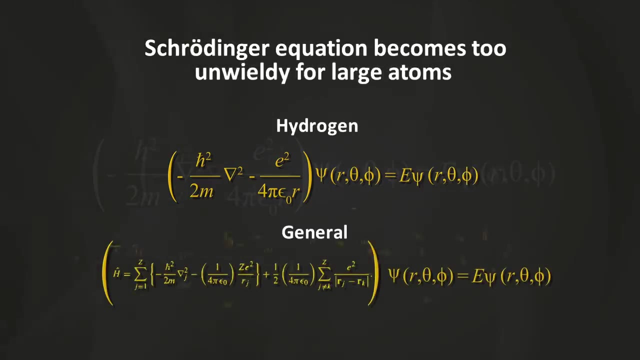 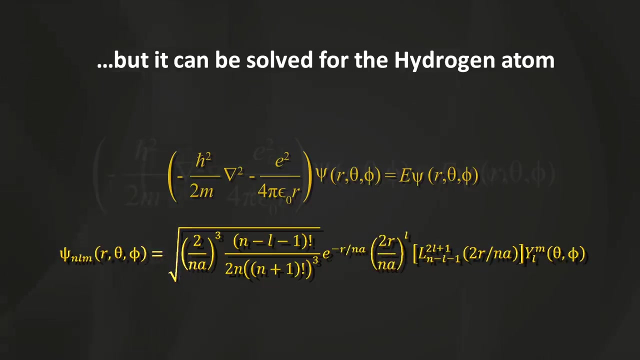 And in those cases the orbits can be occupied in a slightly different way. But the problem is that the Schrodinger equation becomes so unwieldy for large atoms that it cannot be solved. But since we can solve it exactly for hydrogen, it can give us a very good understanding for other atoms. nevertheless, 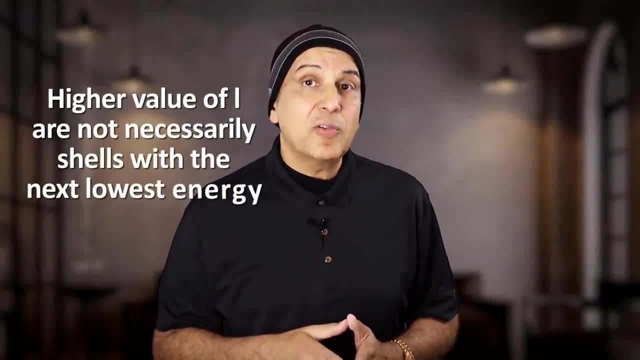 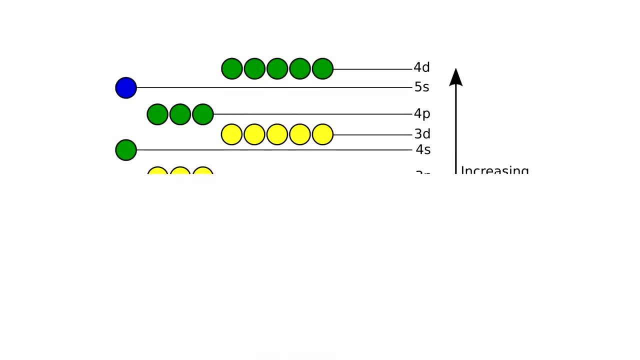 There are also some details that I'm skipping over. For example, you can see that the orbits that are associated with a higher value of L are not necessarily the shells with the next lowest energy. This is why, for example, you learned in chemistry that, instead of starting the d-orbit in the third row, 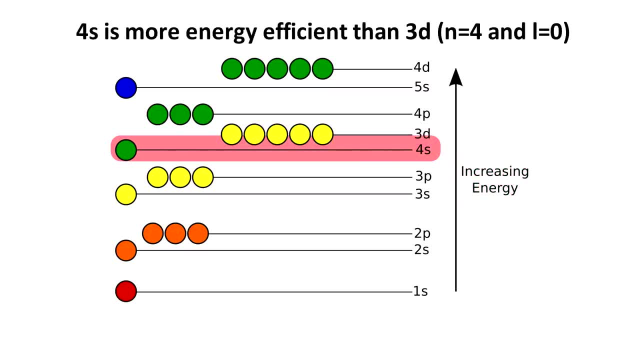 you start with the next s-orbit. The reason is because the Schrodinger equation shows that when n equals 4 and L equals 0 in the s-orbit it is actually more energy efficient than at the d-orbit. But after that it becomes more efficient to fill up the d-orbit. 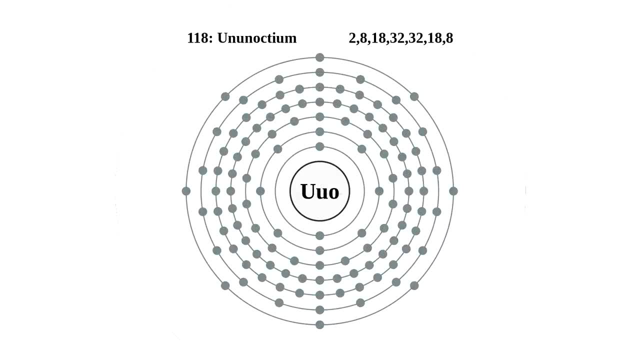 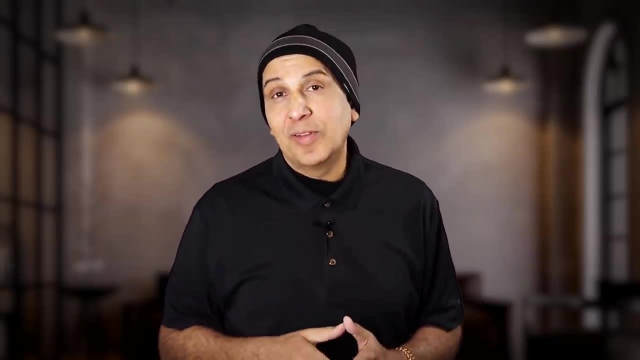 So, simply put, when the quantum numbers of the wave function, you fill up the orbits in terms of what requires the least energy And voila, you get the periodic table. At the end of the day, chemistry is just quantum mechanics with electrons. 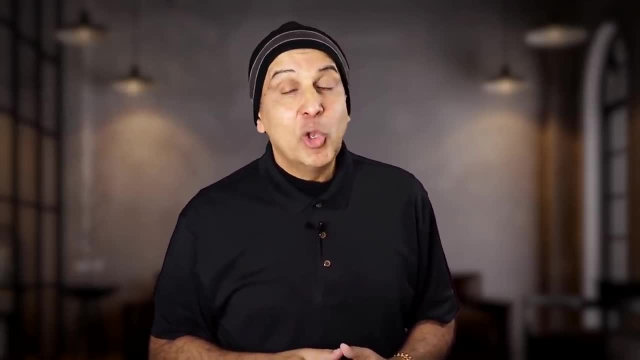 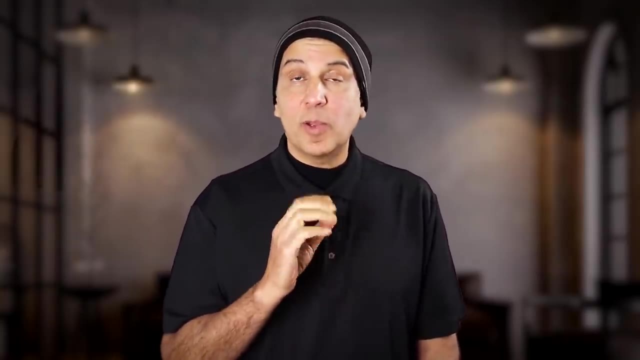 So I hope this helped you finally understand why the periodic table looks the way it does and has to look the way it does. If you want to explore further and learn more about the periodic table of elements, one of the best courses on this subject is available on Wondrium. 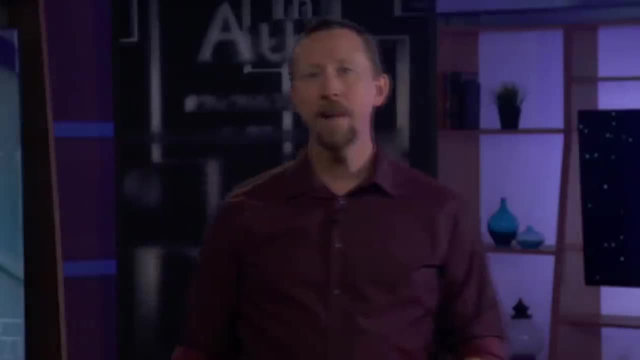 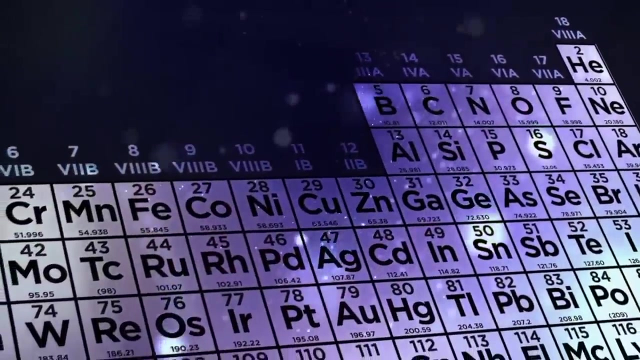 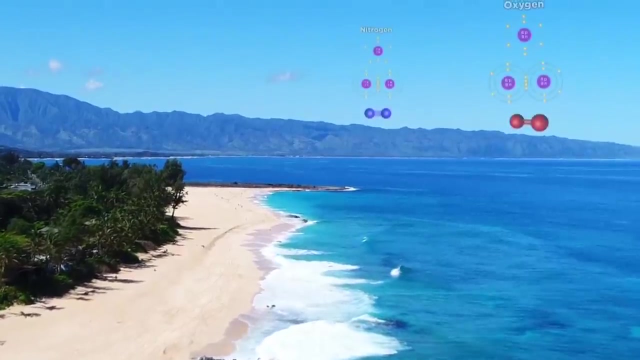 You can get a sponsor called Understanding the Periodic Table, taught by Professor Ron Davis of Georgetown University, His course not only explores the information contained in this iconic chart, but also goes deeper. He answers interesting questions such as: why does neon make for such great lighting? 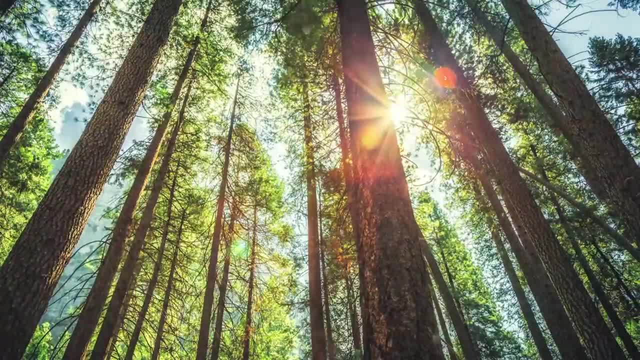 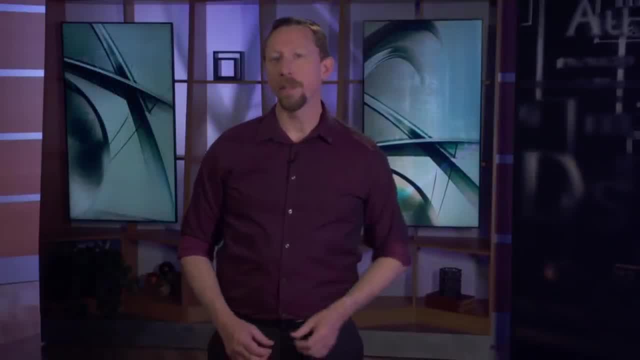 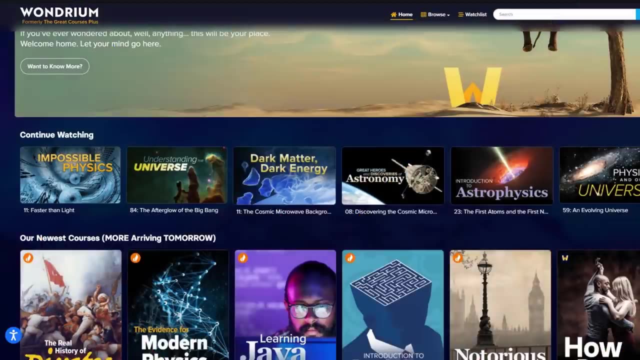 How do nitrogen and oxygen balance Earth's atmosphere for life, And why are copper, silver and gold the colors that they are? You can not only enjoy these great lectures by Professor Davis, but also some of the best educators in the world. You'll be hard-pressed to find a better online learning service than Wondrium. 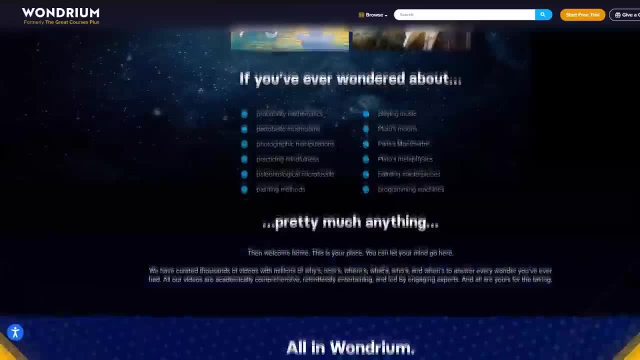 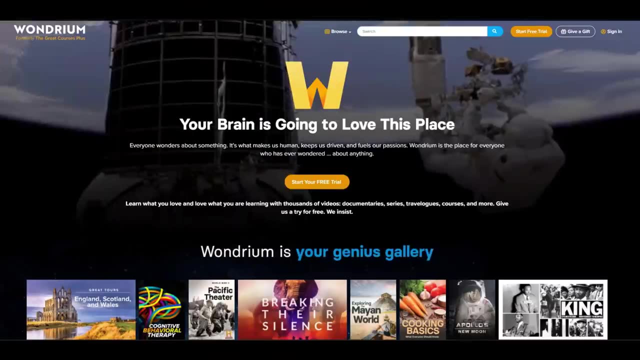 This is why I've been a member for a long time. I couldn't recommend them more. You'll even see my testimonial at the bottom of Wondrium's homepage. It's really easy to sign up right now, because they are offering a free trial. 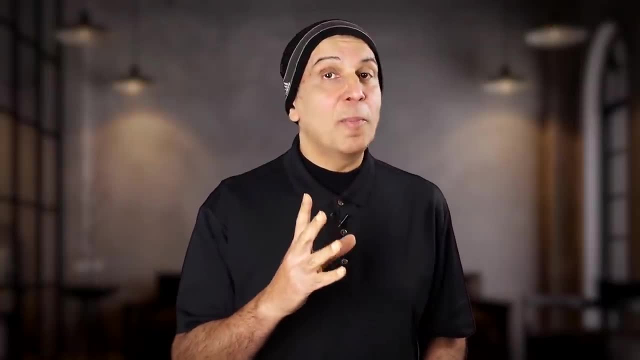 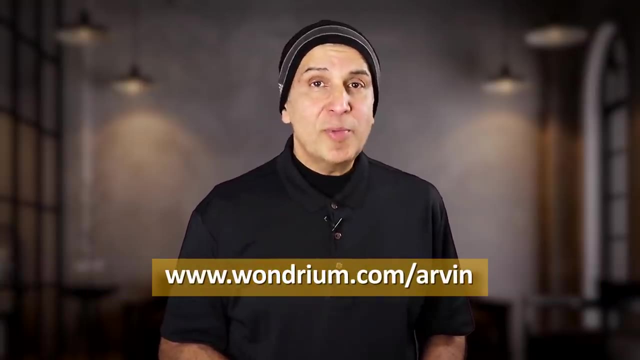 and you can cancel at any time. So you have nothing to lose but a lot to gain. If you want to greatly expand the depth of your knowledge, be sure to click the special link in the description. Wondriumcom forward slash arvind. 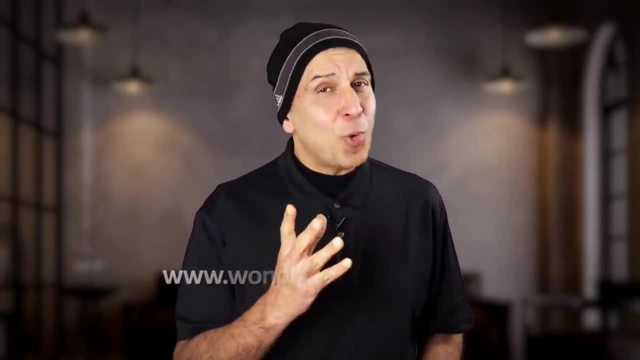 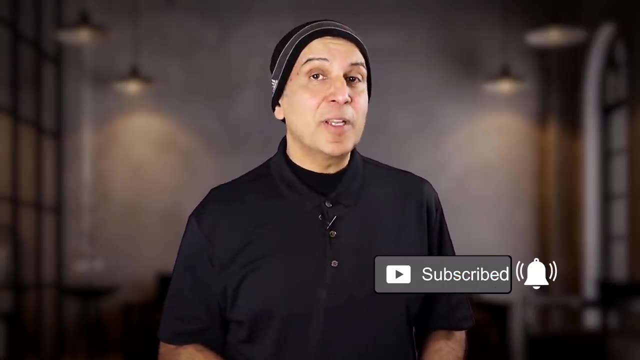 That's Wondriumcom. forward slash, arvind, And you'll be supporting my channel, So thank you for that, And if you have any questions or comments for me or other viewers, please leave them in the comments section. I try to look at all of them.